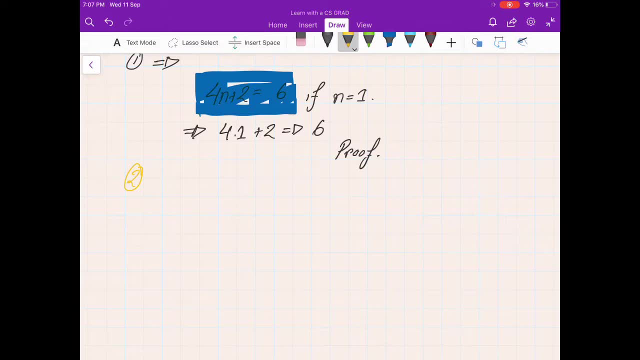 So in proof by contradiction, we try to prove that the opposite or the inverse statement. So the opposite or the inverse statement is wrong, thus proving the actual statement is true. So suppose we have a statement P and we have another statement Q. So this is telling us that if P is going to happen, then Q is going to happen too. 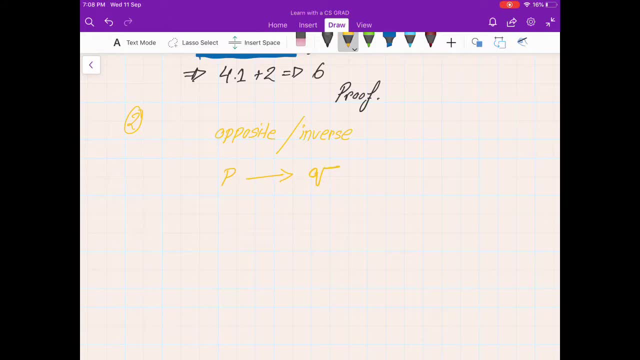 So this is a statement which we have to prove that this is true. So in proof by contradiction, we inverse the statement: So not P equals to not Q, And if this is false, this means that the original statement, that P equals to Q, is true. 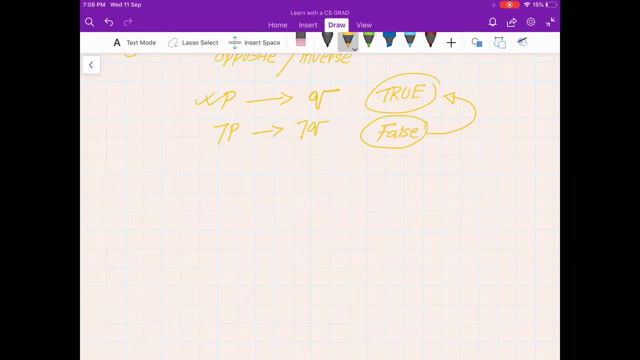 So let's try to understand this with an example. So let there be a statement that if it's 30th Ramadan, then Eid is tomorrow. So here we can see there are two separate statements. If it's 30th Ramadan, let's say this is P. 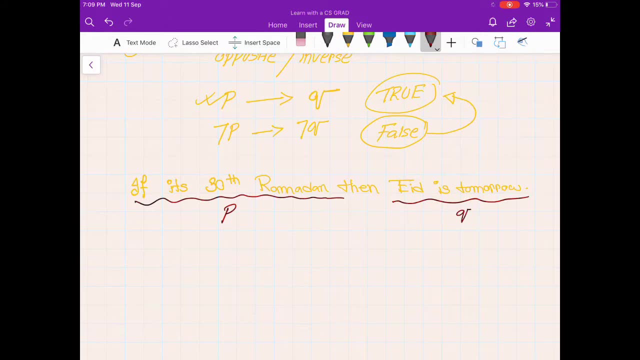 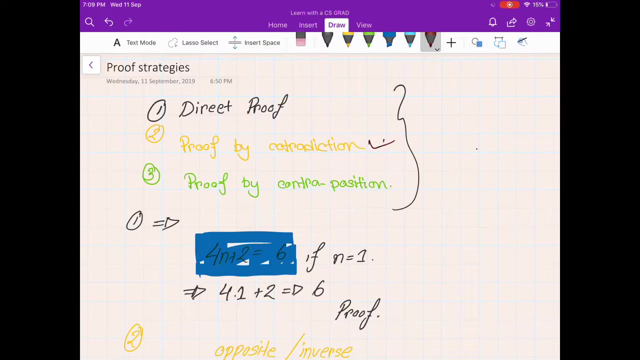 And then Eid is tomorrow. Let's say this is Q Right. And the question asks: prove that this is true. So let's say this is true, And we are trying to prove this using proof by contradiction. So let's try to do that. 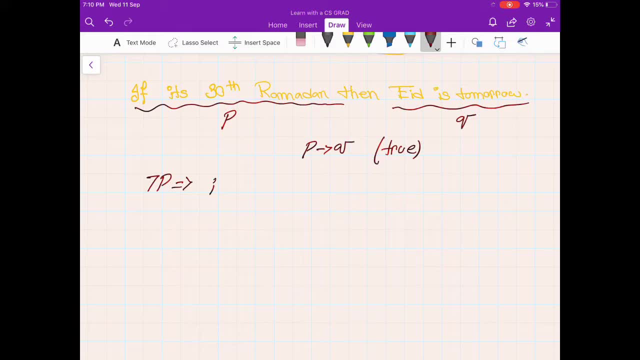 So not P would be. it's not 30th Ramadan. Let's say this is like 29th And not Q would be. Eid is not tomorrow, Tomorrow, Right. So this is false because even if we see the 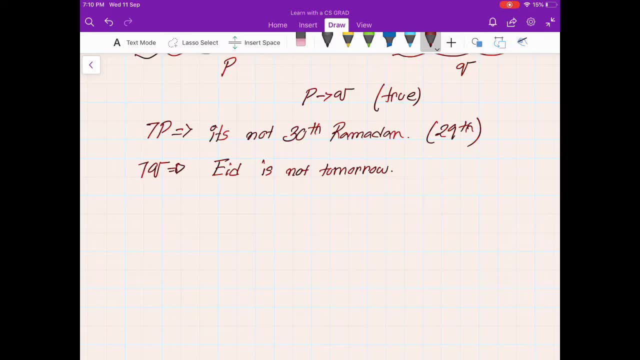 moon on the 29th, then Eid is going to be tomorrow, Right, So this statement becomes false. So not P, not Q would give us a false result, Thus making the original statement: P would would be implication, Q would be true. 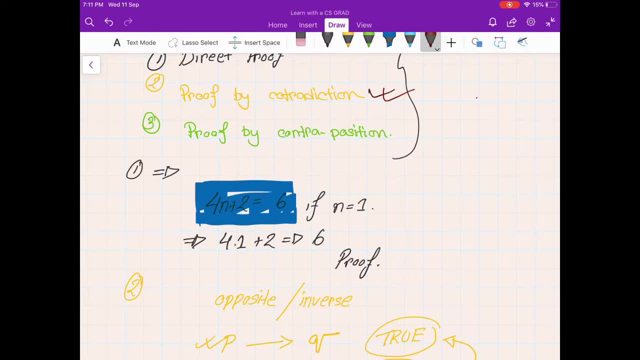 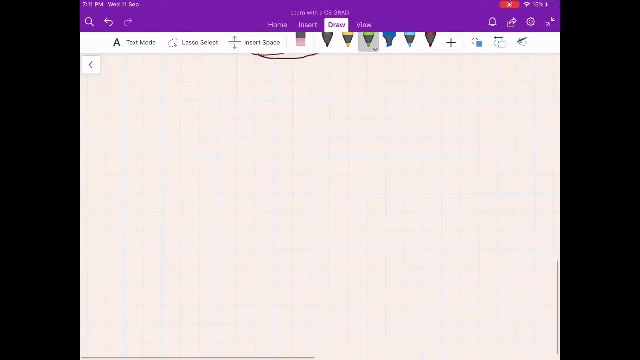 So hope you guys understood that. Let's move on to the third one, which is proof by contraposition. So in proof by contraposition- or we have- we have to remember two things. So contrapositive statement is a combination of two things. 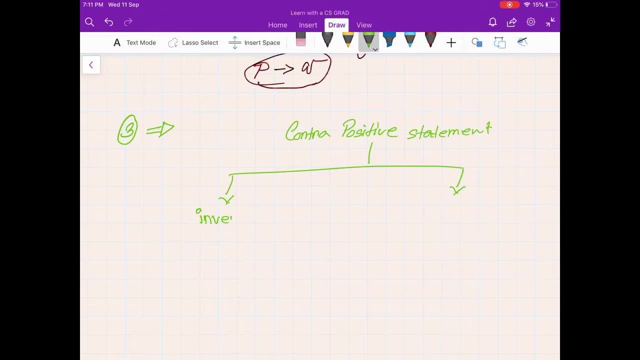 One is: the statement has to be inversed, same as before, And it has to be conversed. So what do I mean by that? So let's assume we have a statement P again and another one Q, So P is 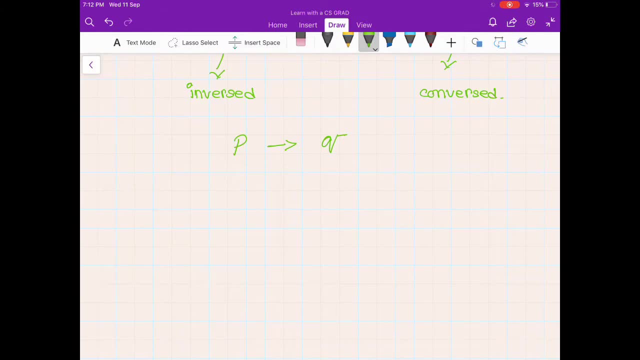 P implicates P implication Q. So what would be the contrapositive statement? It would be: we would inverse it first, So P implicate not, P implication not Q, And then we would inverse, converse it, We would swap the places. 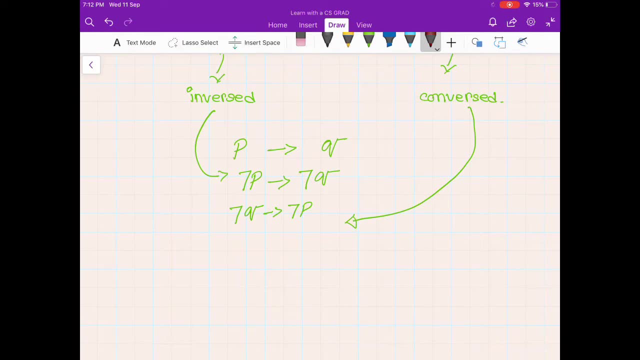 So if we can prove that this statement is true, then the original statement would also be true. So this is different from proof by contradiction, Because here we, after changing the whole statement, we try to prove that it is. 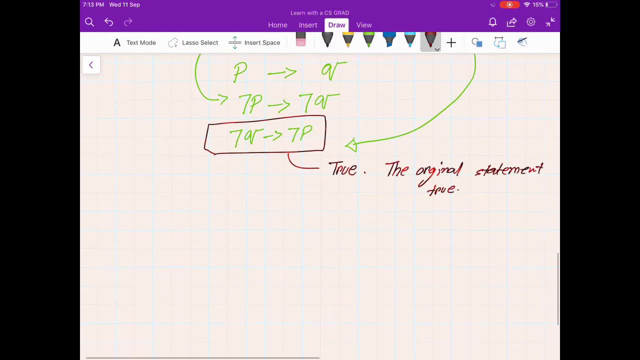 true. So if this is true, the original statement would be true. So let's look at an example here. So let the example be: if 3n plus 2, is odd, then n is odd, Right? 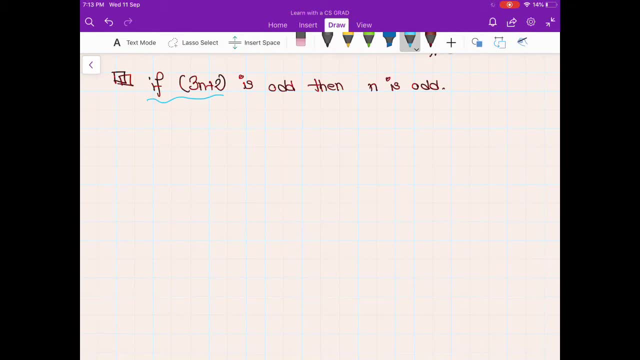 So let's assume that this is P and this is Q. So if you want to prove this by proof or proof by contradiction, I'm sorry if you want to prove this using proof by contraposition. 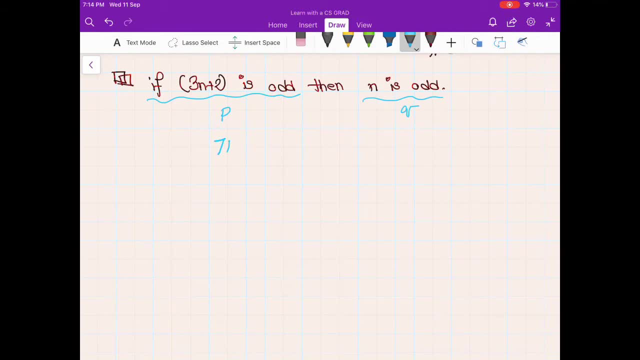 then we would have to first inverse them, then change places. So Q and P? Okay. So not. Q means n is even And not P means 3n plus 2, is. 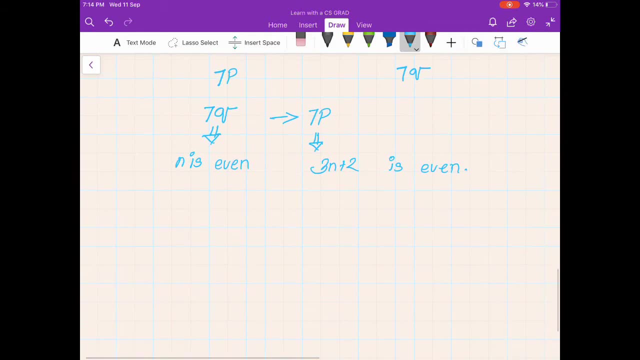 even Right. So let's try to go into the mathematical part here. So 2n is even Right. So then n equals to 2k, Where k is any real number. So. 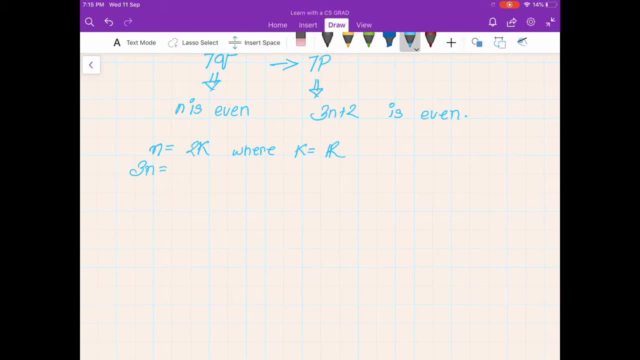 if you try to do 3n, then it becomes 6k. Right, Make sense. And 3n plus 2, becomes 6k plus 2.. Now, now we can take.